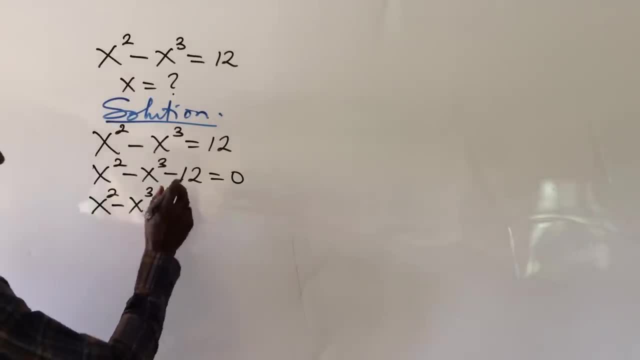 exponents. so if we do that, we can now have this to be s to the power of 2 minus x to the power minus 8, equal to 0.. Now minus 4 or 4 can be written as 2 to the power of 2 and 8 can be. 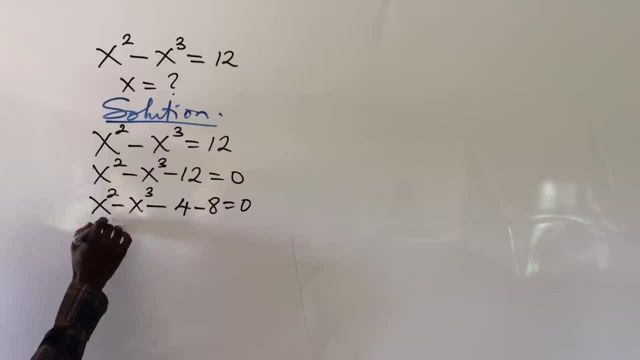 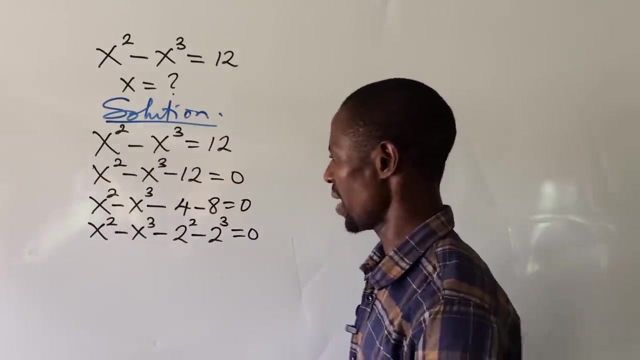 written as 2 to the power of 3.. So we now have this to be x to the power of 2 minus x to the power of 3 minus 2, to the power of 2 minus 2 to the power of 3 equal to 0.. Very easy, So we are. 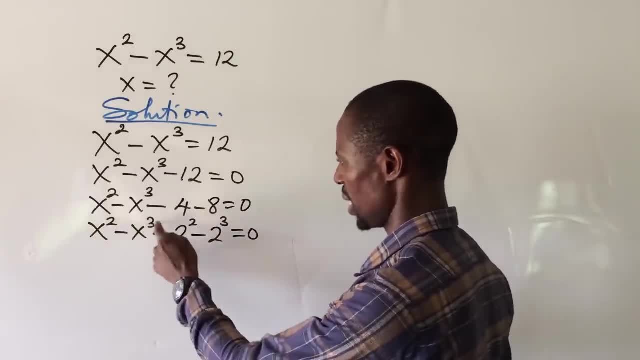 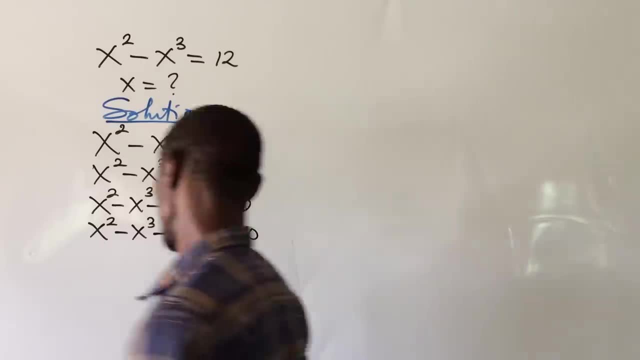 having 2 to the power of 2, we are having x to the power of 2, x to the power of 3, 2 to the power of 3.. So we can bring this and this together. bring this and this together. Okay, so if we do that, 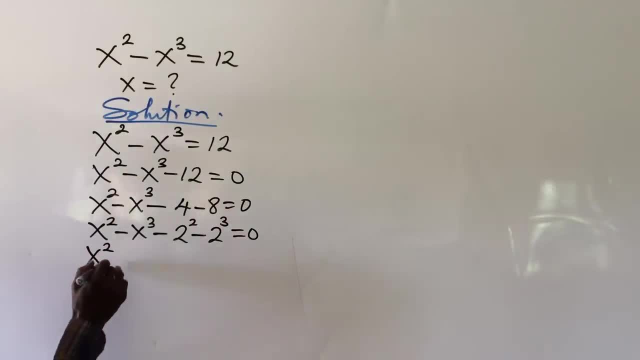 we're going to have this to be x to the power of 2, then minus here, 2 to the power of 2, minus x to the power of 3. bring this together with this: 2 to the power of 3, equal to 0.. This is simple. 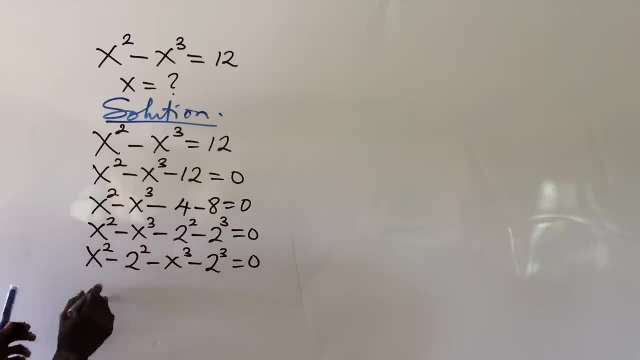 Okay, So we can go ahead and group this, group this. So we now have bracket open x to the power of 2 minus 2 to the power of 2 goes bracket minus. bracket open x to the power of 3 minus 2 to. 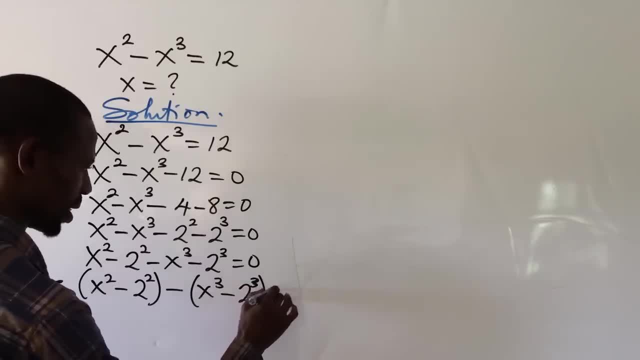 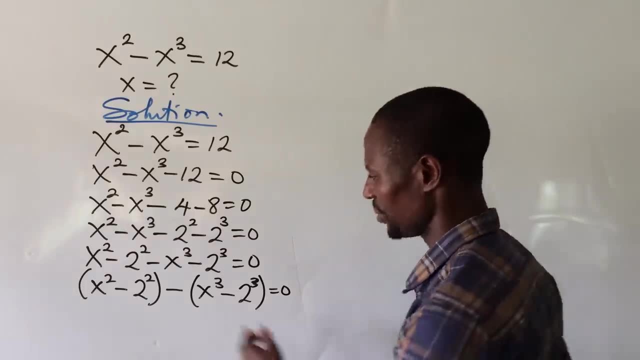 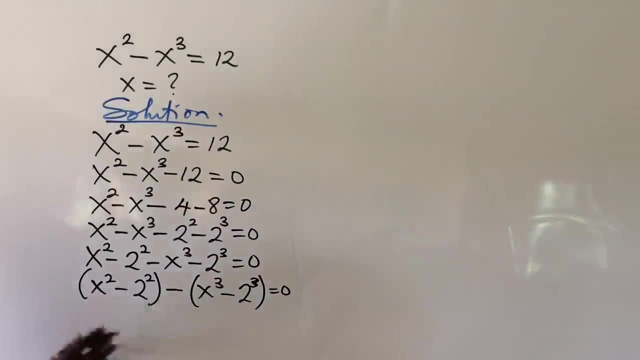 the power of 3.. Okay, Those brackets are equal to 0. Okay, Very easy. Now, mind you, here we are having a minus sign, So we can use this minus to bring up this bracket here. So if we go ahead to do that, we're going to have here to be bracket x. 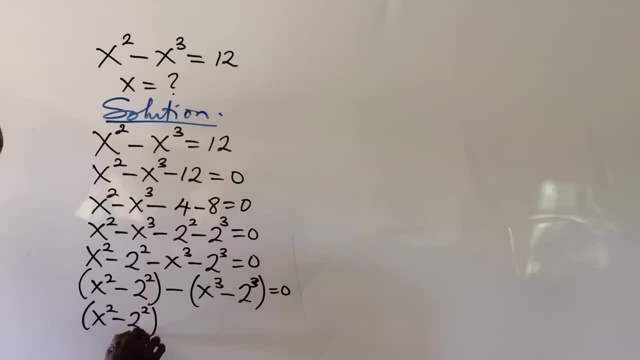 to the power of 2 minus 2 to the power of 2 goes bracket minus bracket. x. to the power of 3 plus 2 to the power of 3 goes bracket or equal to 0.. So let's proceed from here now. 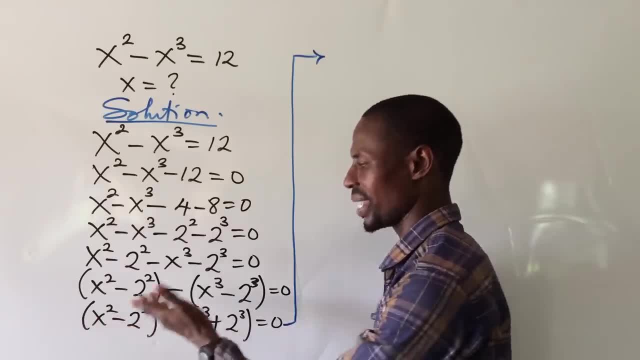 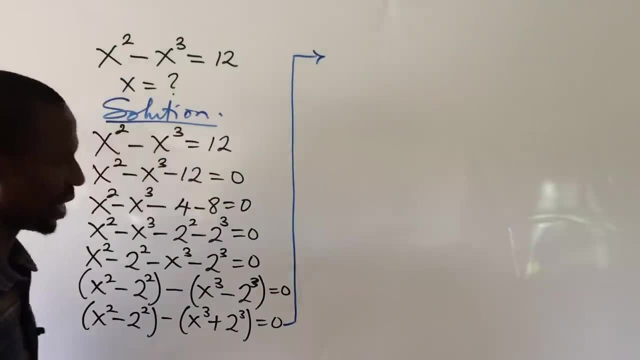 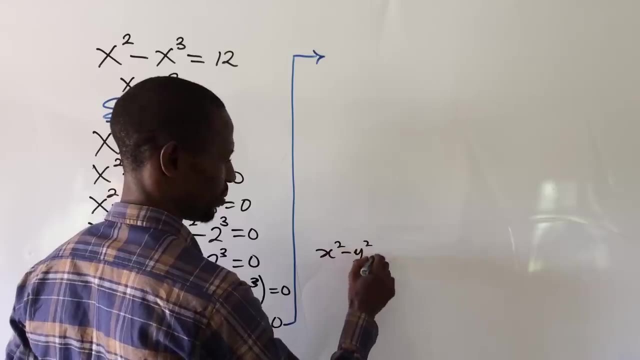 If you take a look at this, we have some special algebraic identity playing out already. Now let's cast our mind back and bring up the algebraic identity. Here we have your s to the power of 2 minus y to the power of 2.. This is 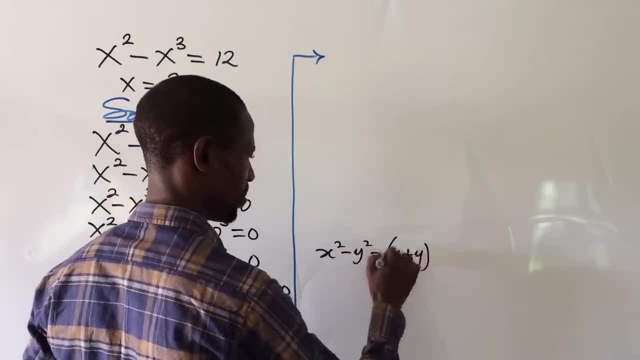 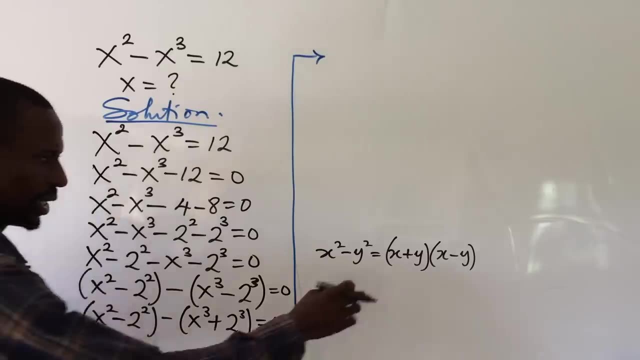 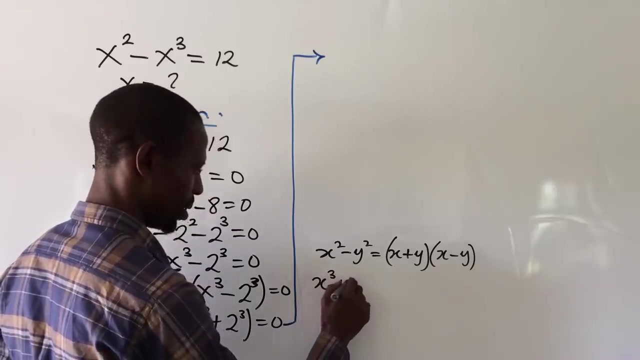 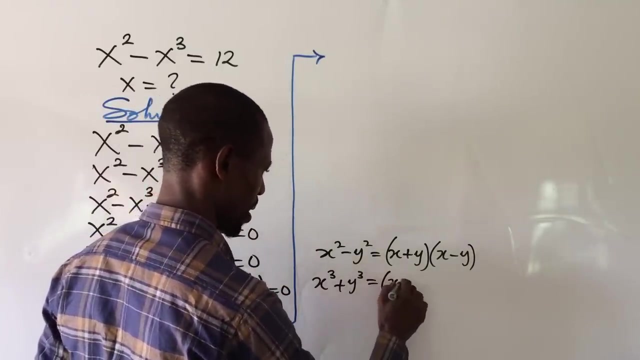 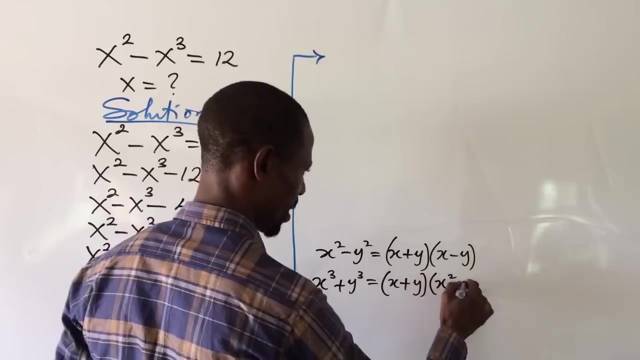 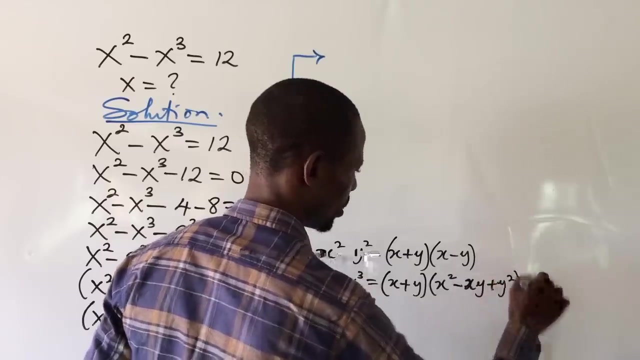 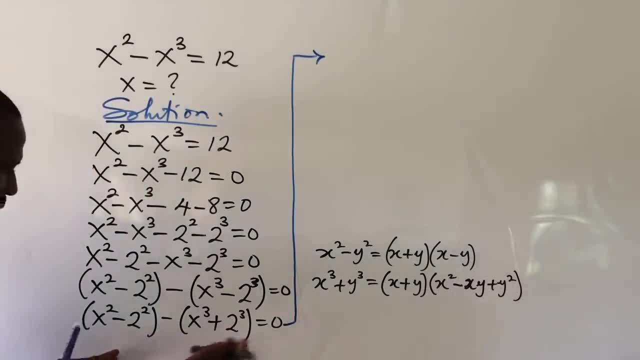 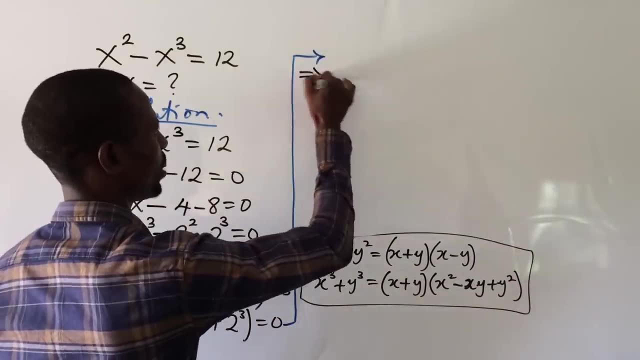 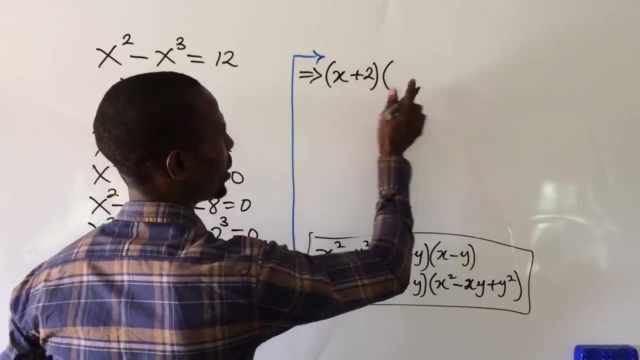 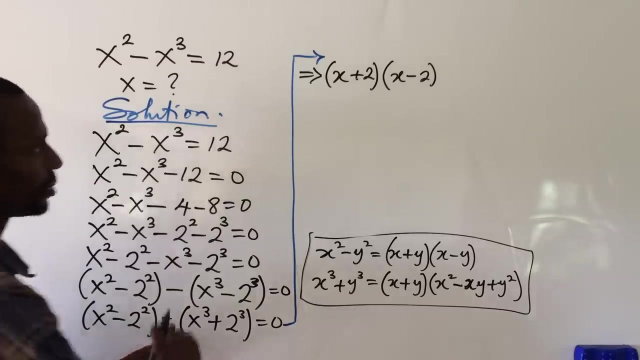 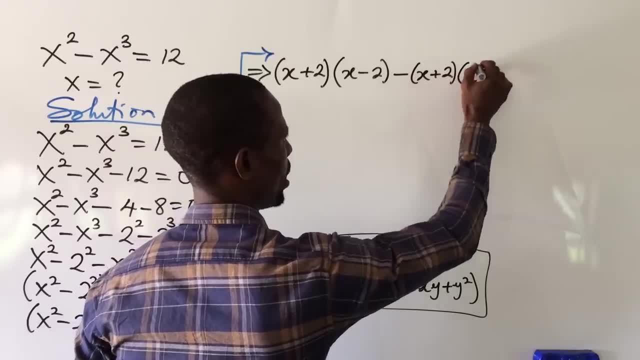 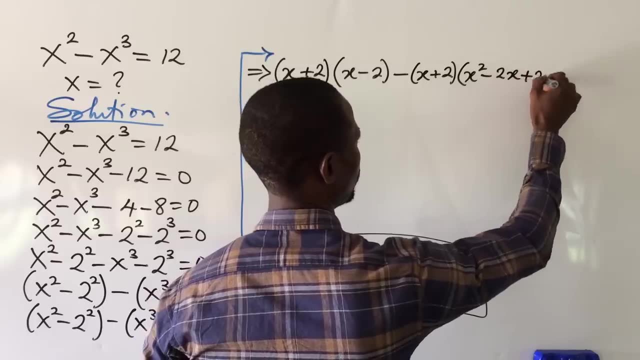 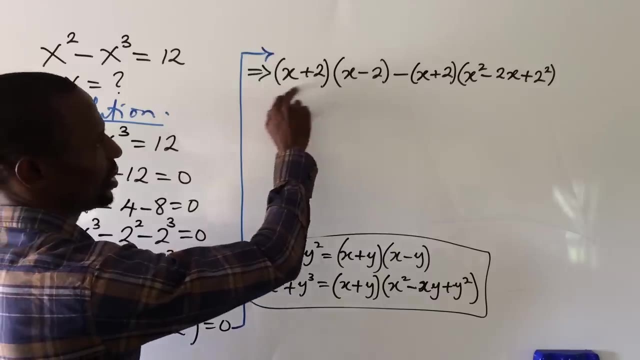 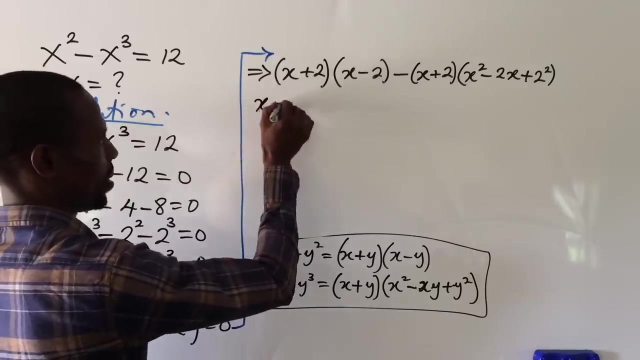 plus two close bracket. bracket your s squared, then minus your two s plus your two to the power of two close bracket. okay, then from here, what we do? you look at this: we are having x plus two here, we're having x plus two here, so we can factor that out. so if we do that- and i have this to be s plus, 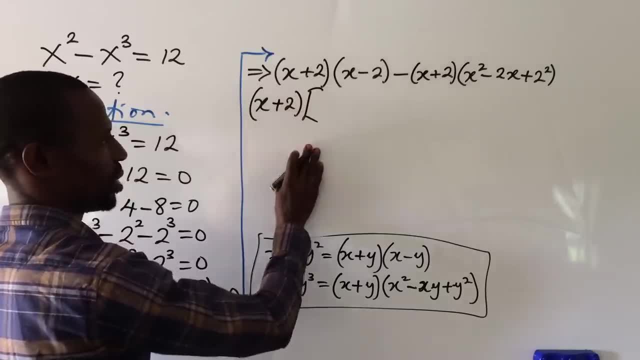 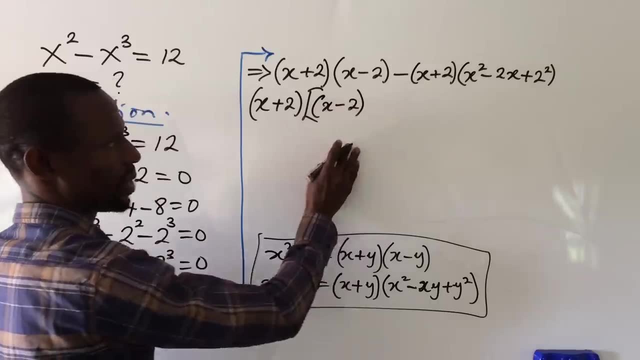 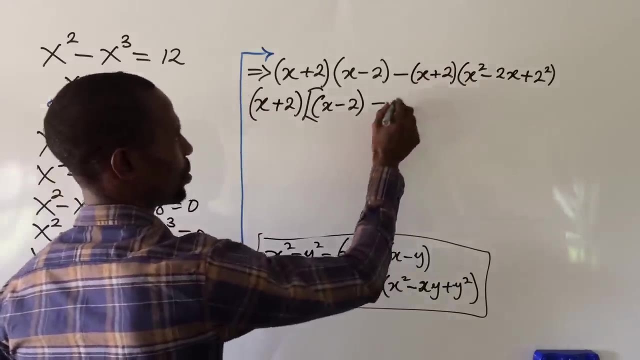 two to be factored out into our square bracket. if you use this to divide everything here, you are left with your s minus two. close bracket, then minus. if we use this to divide everything here, this will leave and you are left with this. so we now have your bracket x to the power of two. 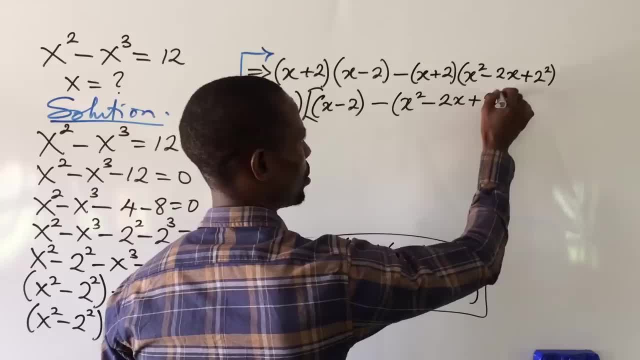 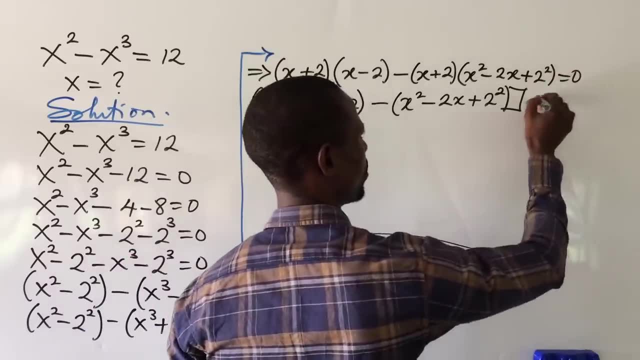 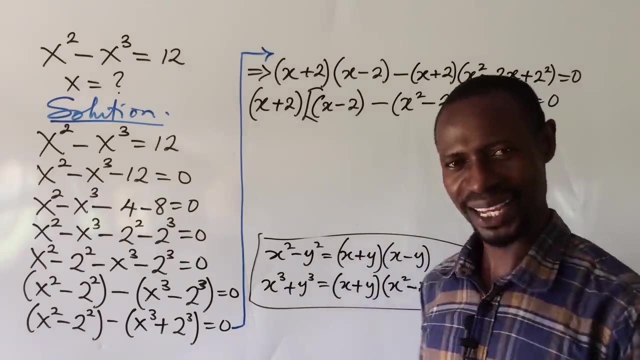 minus two, x plus two to the power of two close bracket, or it's our square bracket. do not forget, we have our zero on the right hand side of the equation. any confusion so far? no, but before we continue again, if you are new to this channel, do not forget to subscribe and share with your 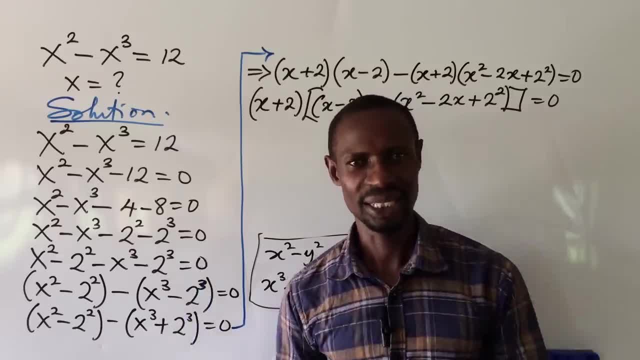 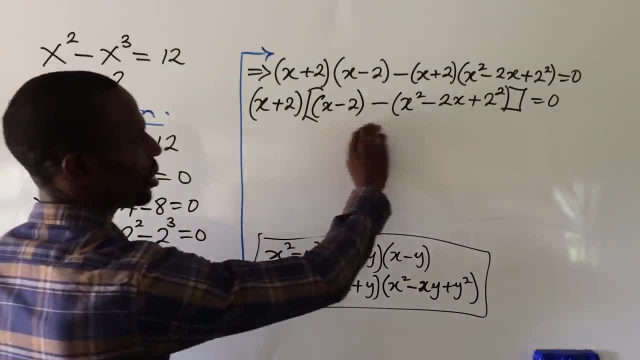 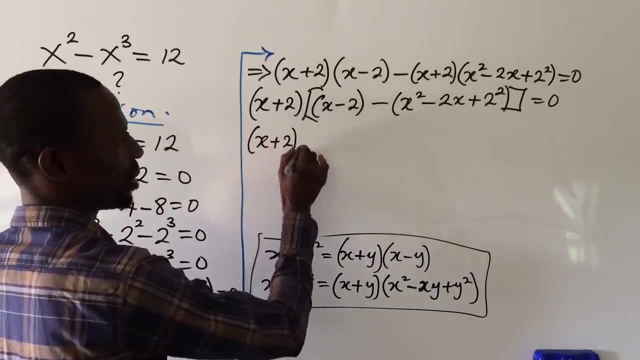 friends with your family members that need this knowledge. okay, let's go back again here. we cannot open up what we have inside the square bracket now. if we do that, we will come out with you plus two brackets. open then bracket, you will go to have s minus two, then minus. 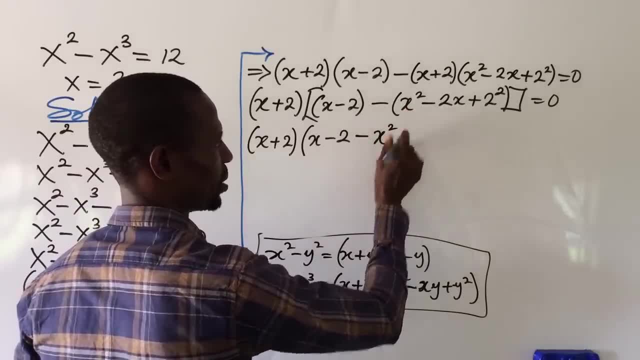 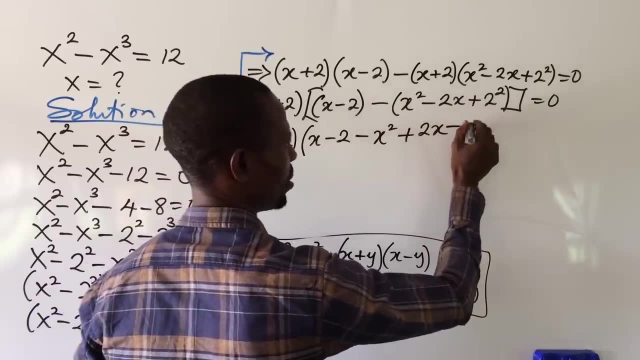 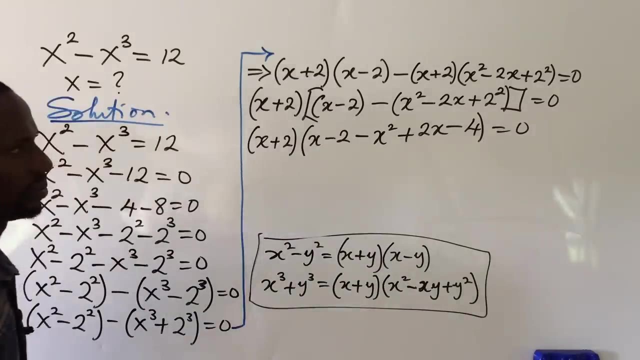 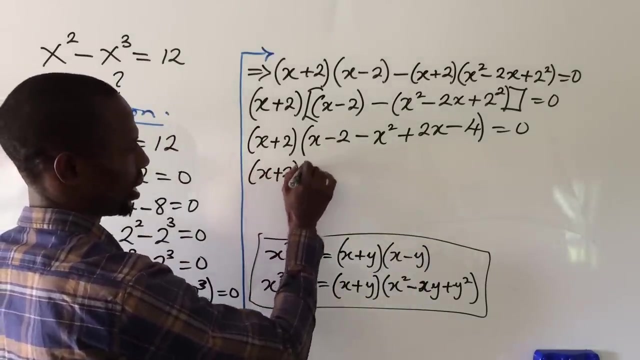 minus times this plus x square will give us yeah, minus x square. minus times minus will give us plus two. s minus times plus will give us minus two to the power of two will give us four. those brackets are equal to a zero. good, so let's work on what we have here now. so we have s plus two bracket bracket. 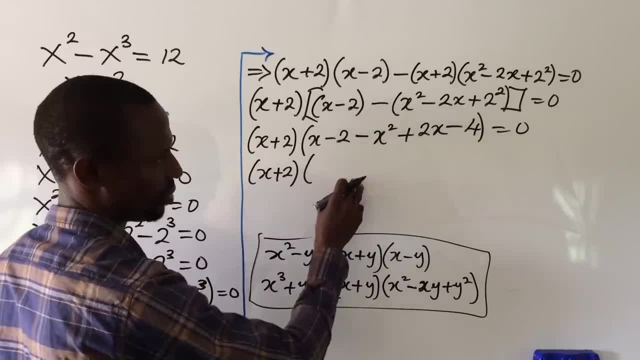 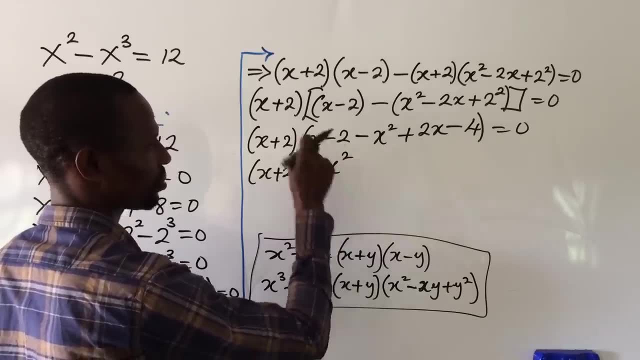 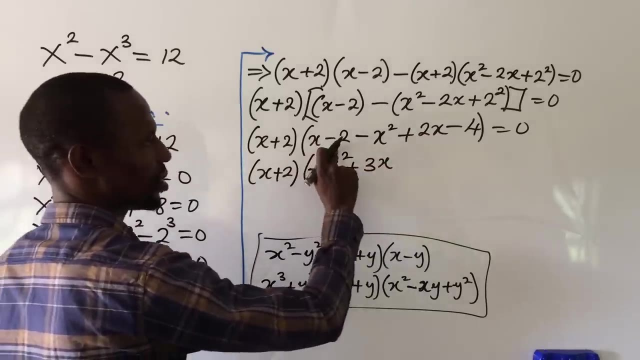 let's hold. let's bring this minus x to the power of two out first, because it's the one with the highest variable. so we have this will be minus s to the power of two. plus x plus 2s will give us plus three. x minus two minus four will give us. 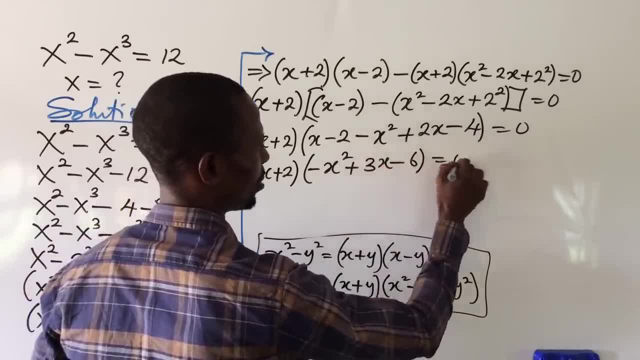 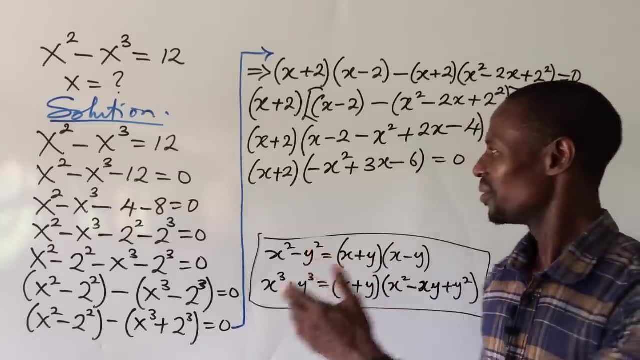 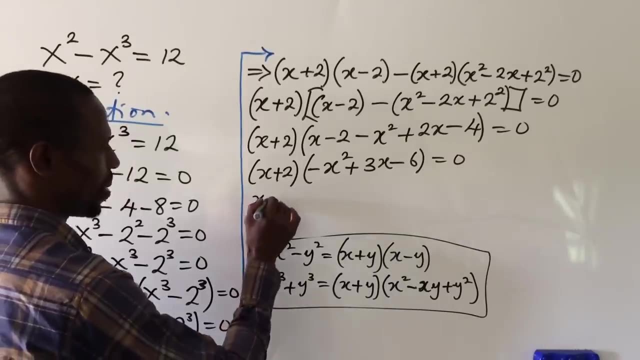 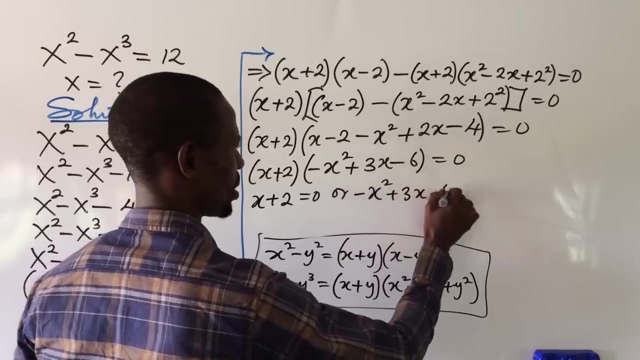 my minus six equals bracket or equal to zero. okay, at this point we succumb to the zero product rule, whereby we equate this to zero. equate this to zero. so if we do that, we're going to have here s plus two equal to zero, or minus s to the power of two plus three s minus six equal to zero. good, 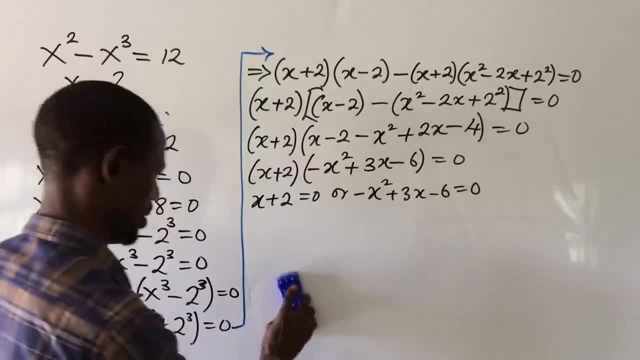 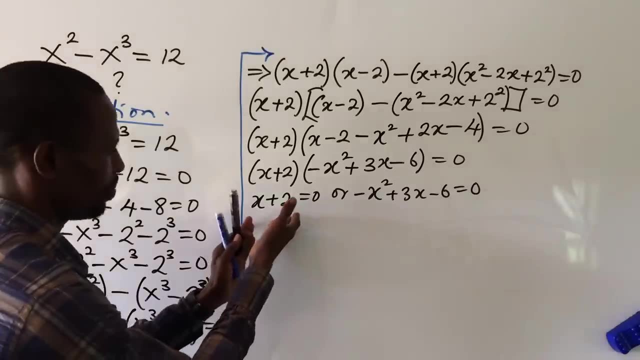 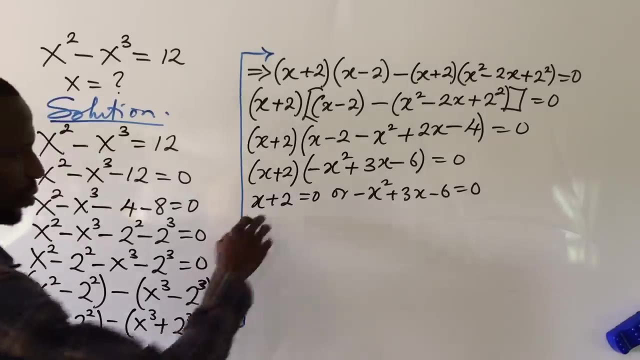 let's erase this. this is our identity. we are done with it. okay, we look at this again. we don't have problem with this side of the equation, okay, we only have some little challenges with this other side. so this: we send this to this side to give us here s equal to minus two. automatically, we'll go. 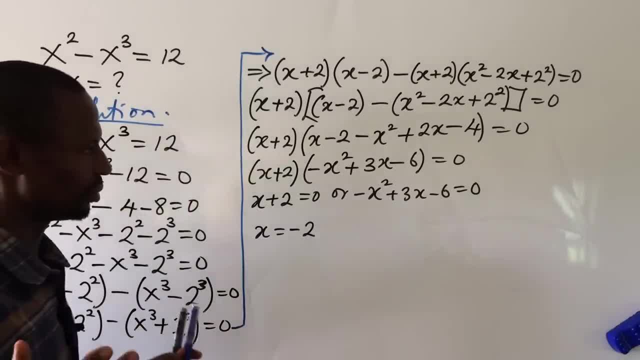 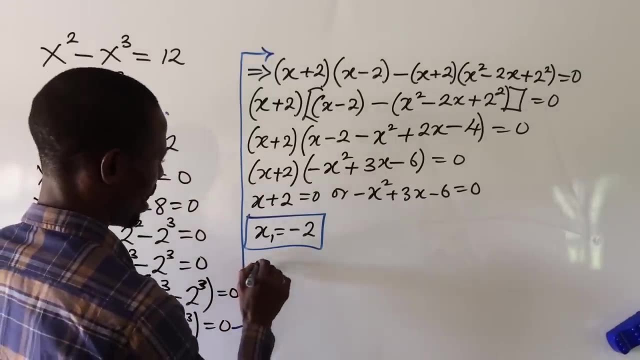 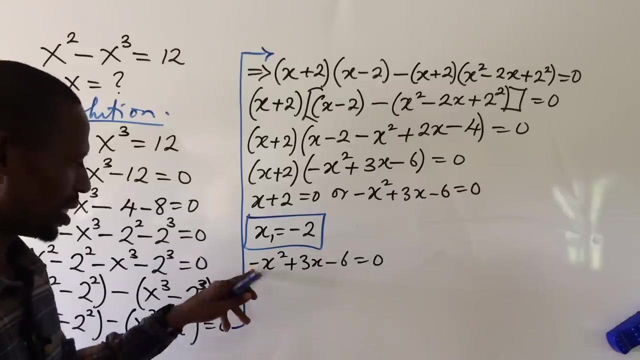 the first root. okay, to our challenge already. so let's give this the the the first truth: x1. this is the first root. we cannot handle this side of the equation now. this: we have this to be our minus x to the power of two plus three s minus six, equal to zero. we can eliminate. 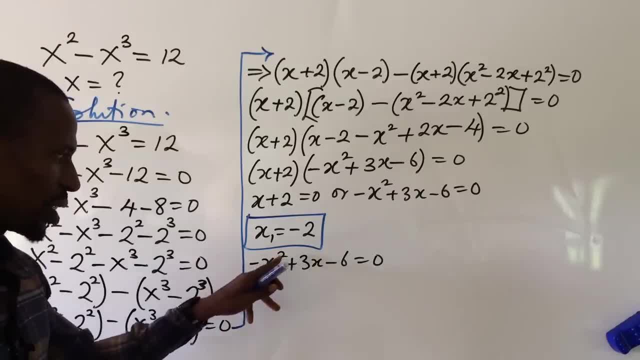 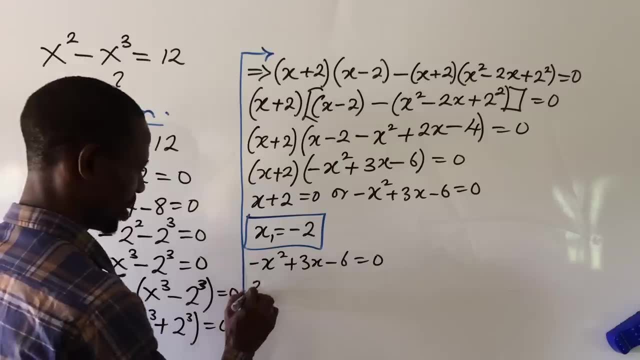 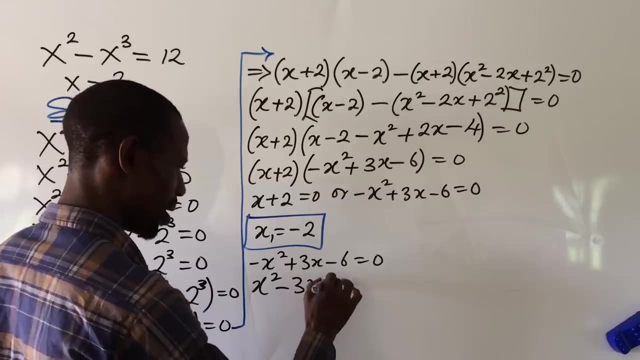 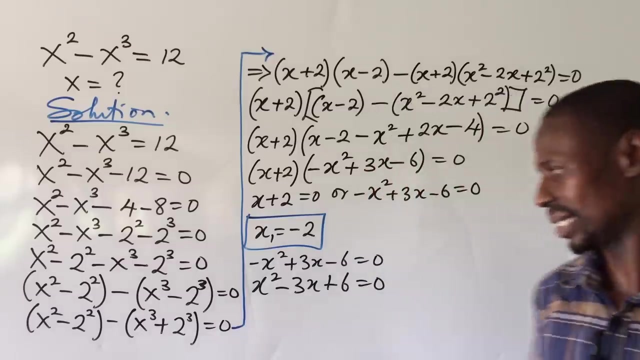 this minus one attached to this s square by multiplying all through by a minus one. okay, and so this will now give us a x to the power of two positive minus three s there plus six, equal to zero. automatically, this is a quadratic equation, so we solve this quadratically, okay. 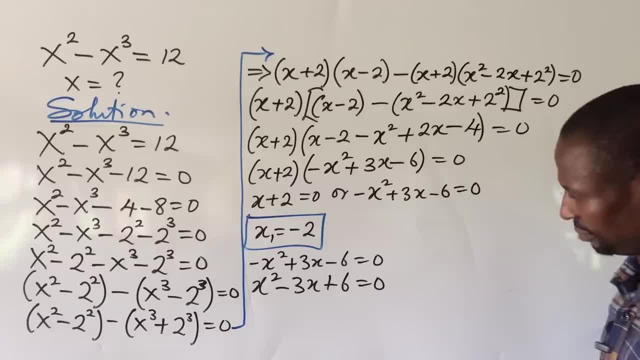 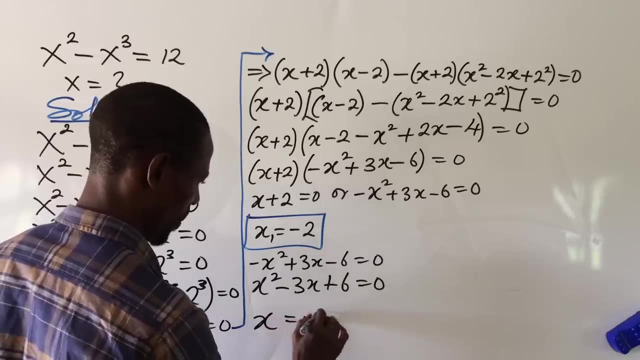 now, solving this quadratically, you discover that, um, we cannot use the factorization method. okay, so we succumb to the formula method. so, using the formula method, the formula method says, um that x is equal to your minus b plus minus the square root of b, squared. 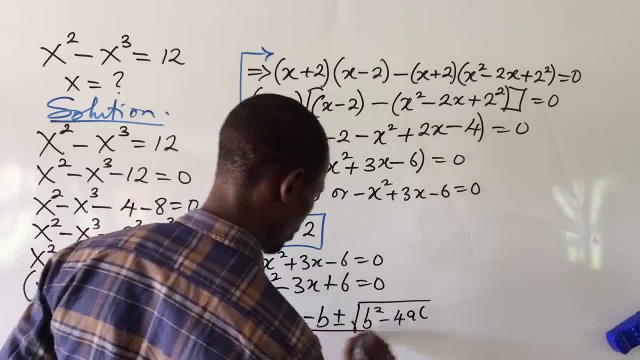 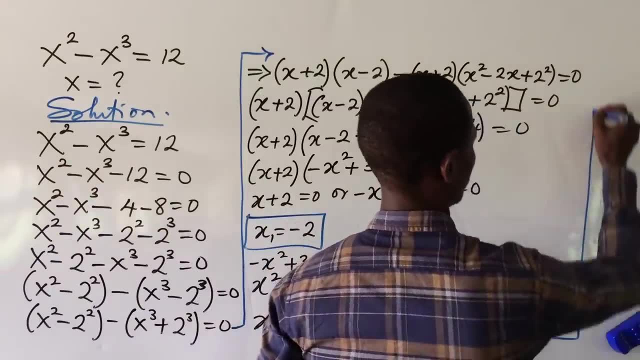 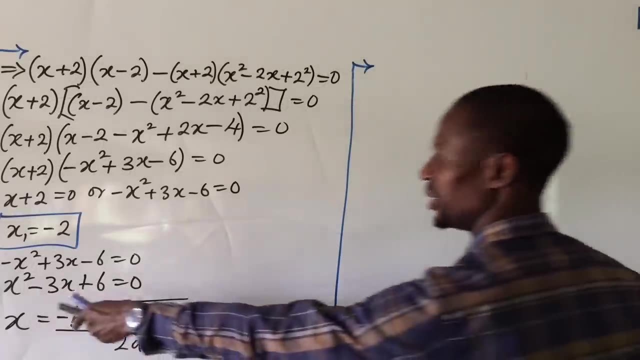 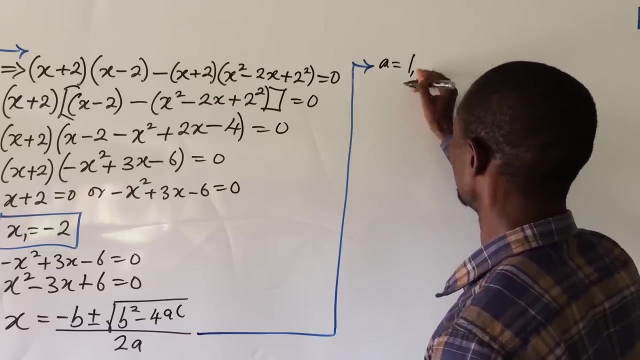 minus four e, c all over to a again. let's proceed from here. all right now, let's figure out our a, b and c from this uh equation here now. so from here we have our a equal to: the coefficient is one, the comma, the b is equal to um. 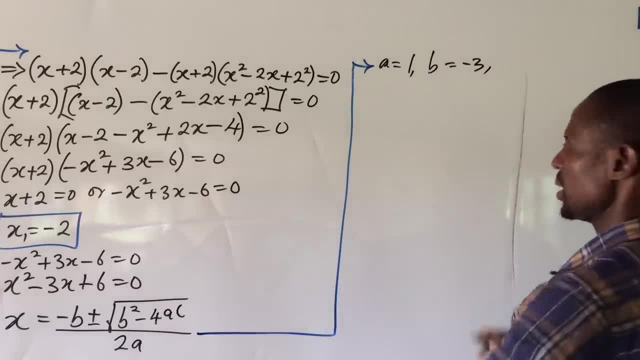 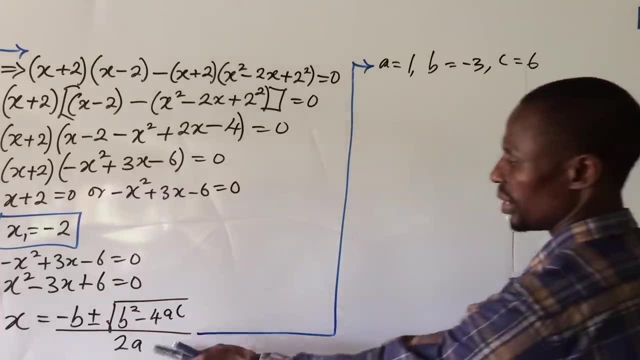 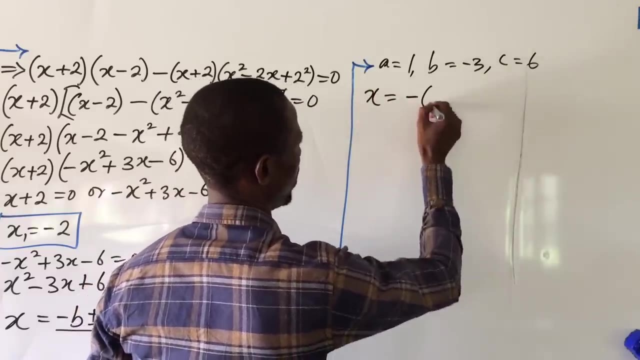 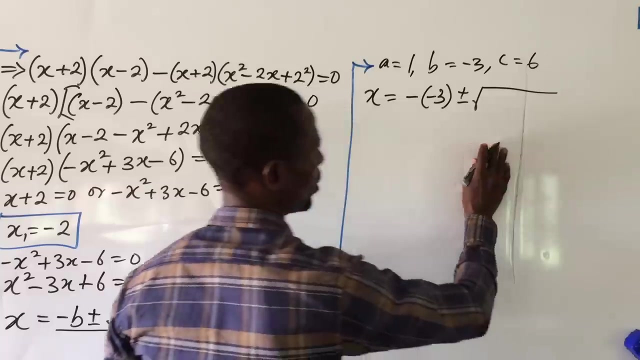 minus three. the c is the constant term, which is six. okay, so we cannot go ahead and substitute this into our quadratic formula, so we're gonna have this to be our s equal to minus bracket. our b is minus three, minus three plus bracket, plus minus the square root. 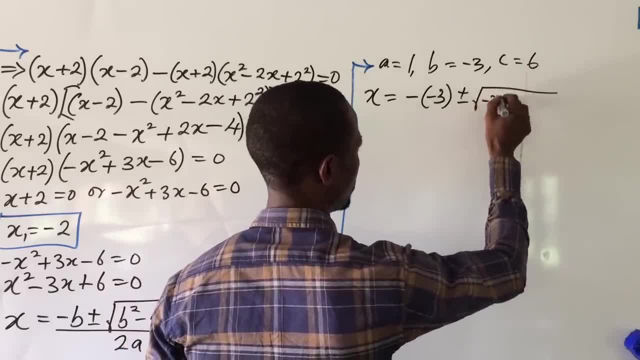 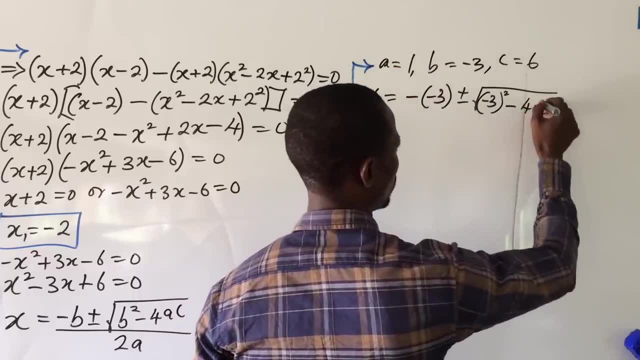 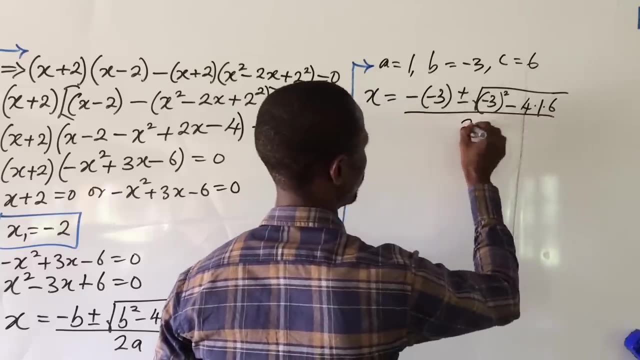 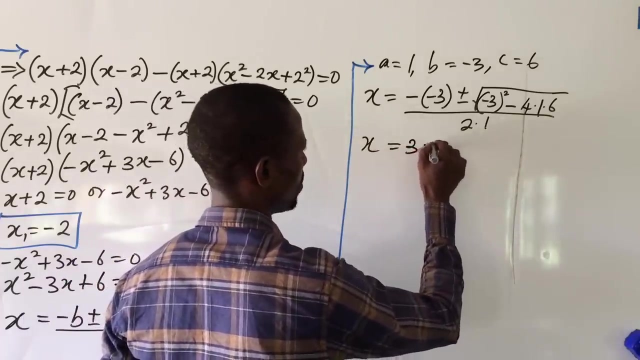 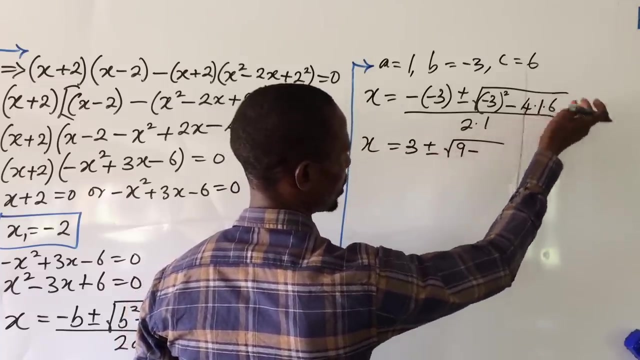 of what is our b, again minus three, out of the power of two minus four. dot what is our a, one dot our c: six. everything all over two dot one. so we have our s equal to here. we have positive three plus minus. the square root of nine minus four, multiplied by one times c's will give us 24.. 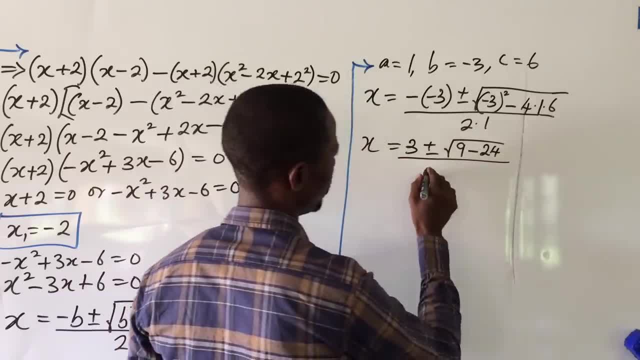 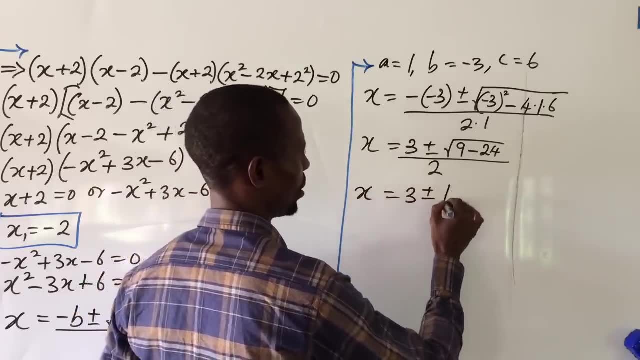 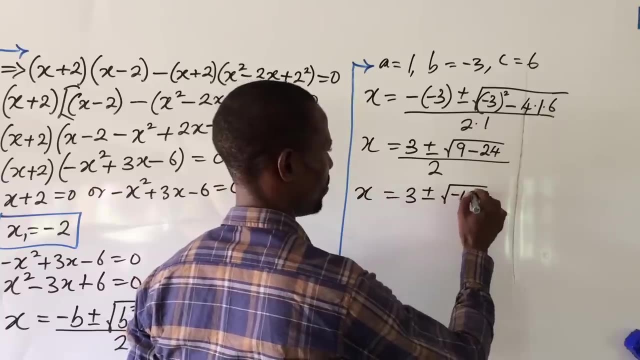 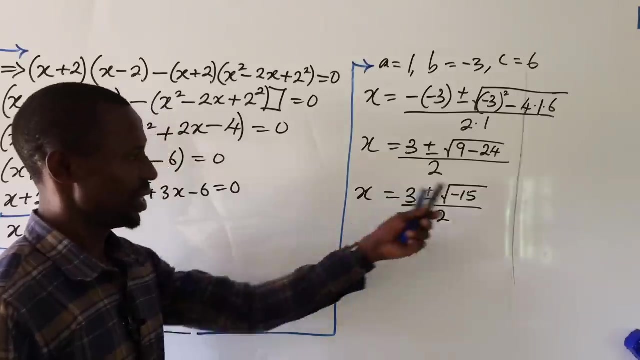 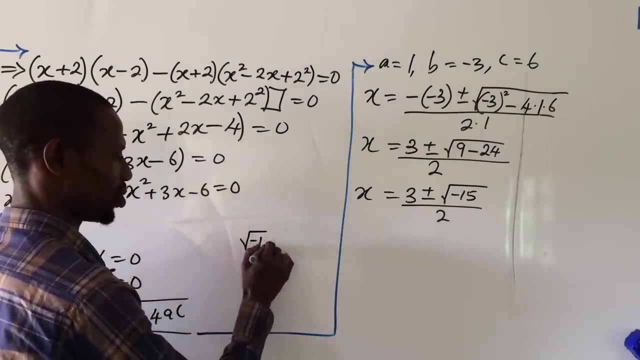 okay, yeah, everything all over your two. yeah, we don't have this. x equal to three plus minus the square root of nine from 24 will give us minus 15 all over two. okay, yeah, remember the identity which says that if you have your r and we say that root minus one equal to your imaginary number i. 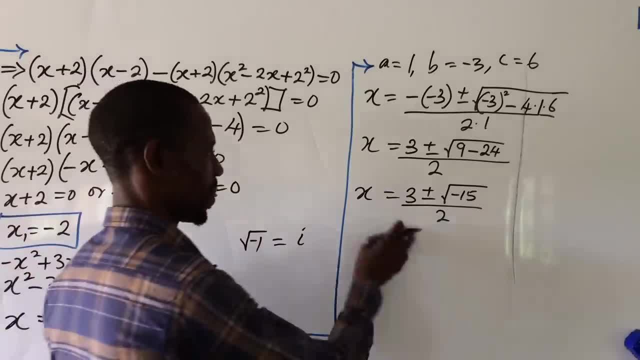 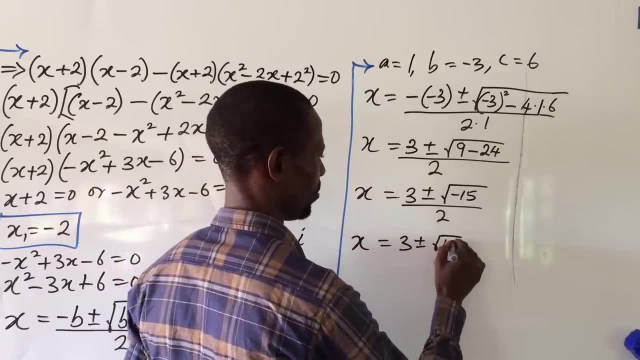 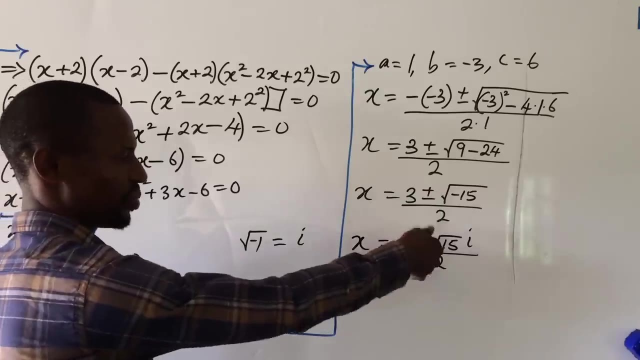 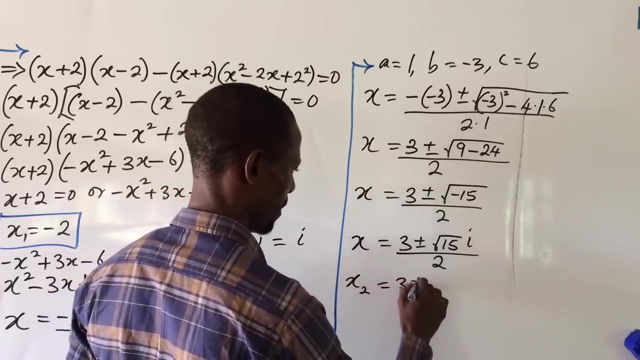 so we can split that and bring out this identity here, and so this will not give us x equal to three plus minus the square root of 15, i all over 2. we have two roots here now, so we can split them out to give us here our s2 equal to your 3 plus. 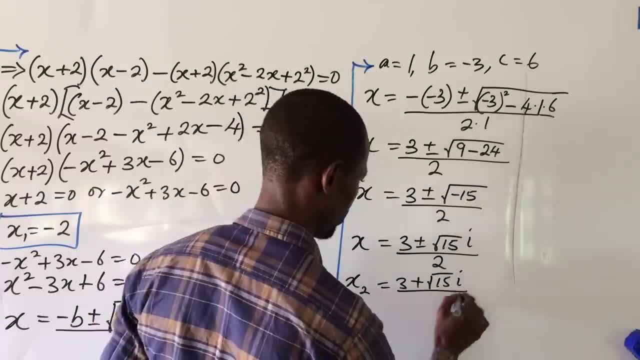 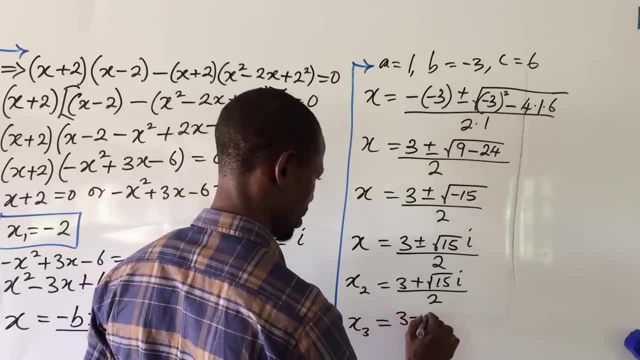 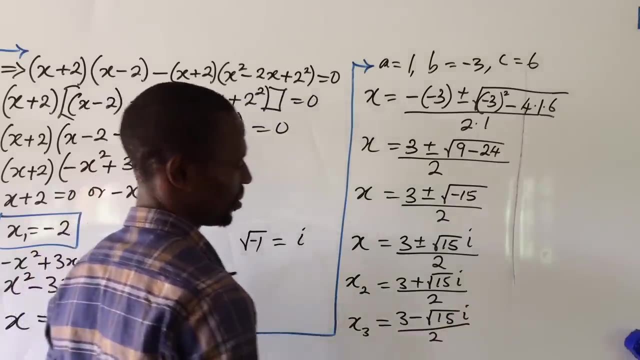 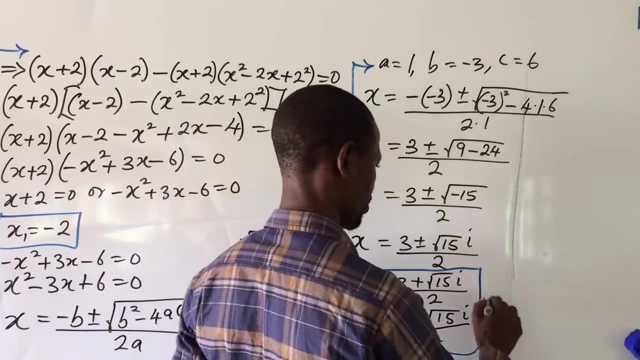 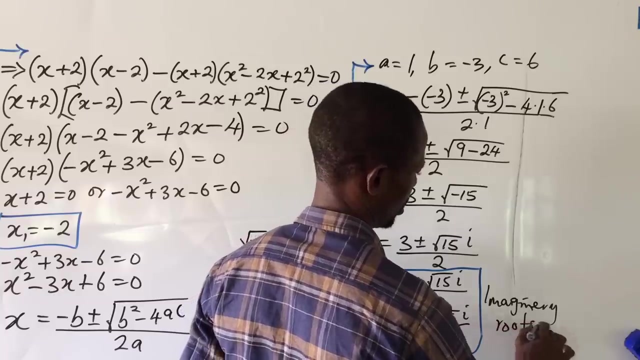 root 15, i all over 2, and your s, the s3, equal to 3, minus the square root of 15- i all over 2. okay, so these are the other two roots. so these are the imaginary roots. so this challenge imaginary roots, these are the imaginary roots. now we can equally check. 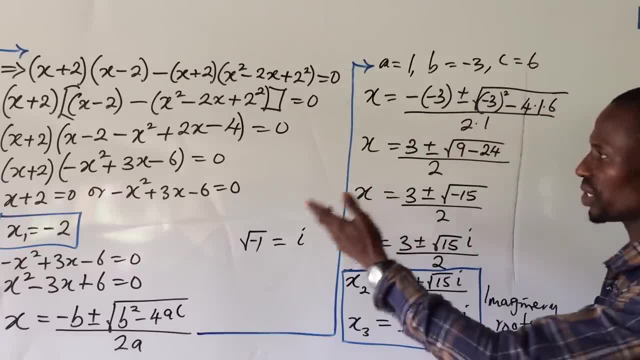 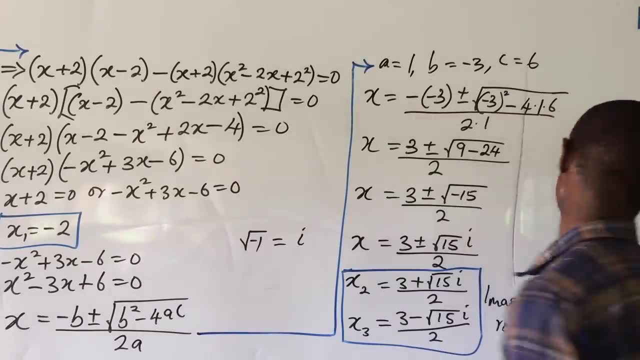 if our answer is correct, if you plug in the first answer, which is minus 2, into our system- minus 2 into our system- you're going to get the correct answer. but let's check our real root. we have our s1 equal to minus 2 and our question is: your s to the power? 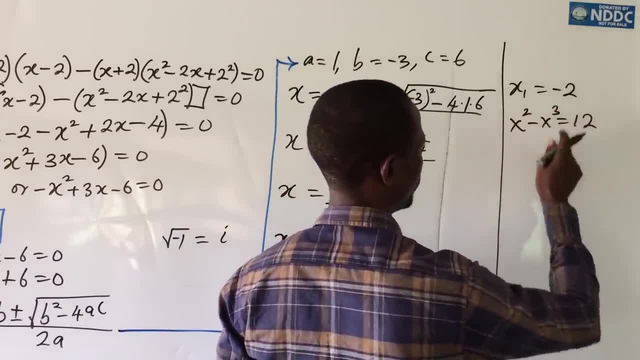 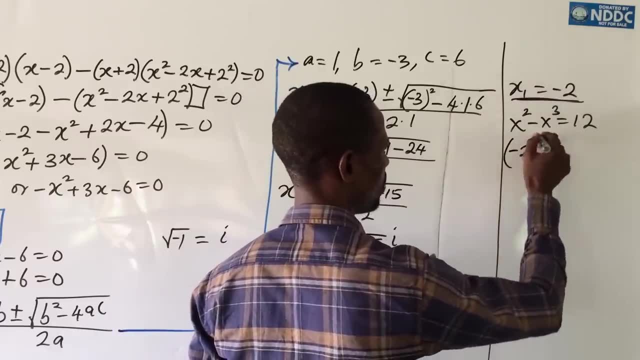 of 2 minus s to the power of 3, equal to 12. so wherever we see your s, we put in minus 2, so we have this to be minus 2 out of the power of 2, minus bracket, minus 2 out of the power of 3. 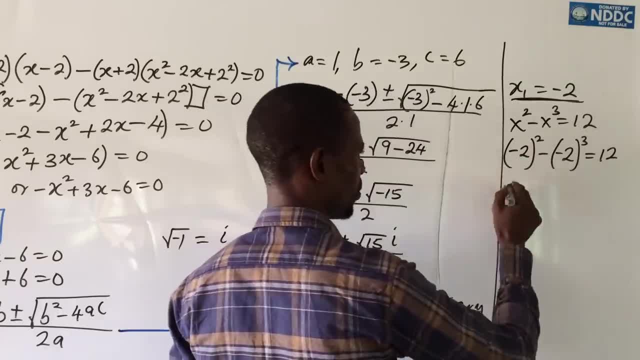 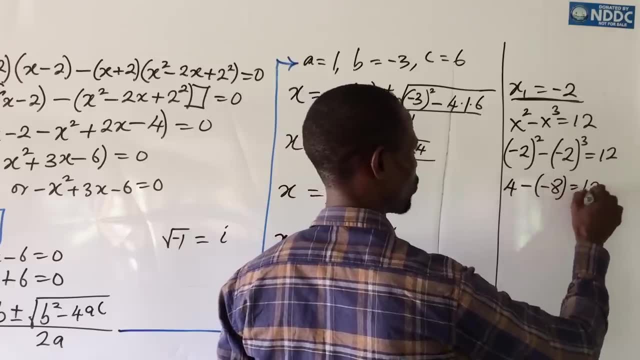 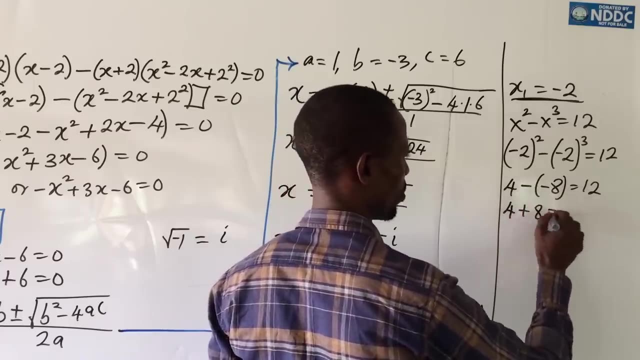 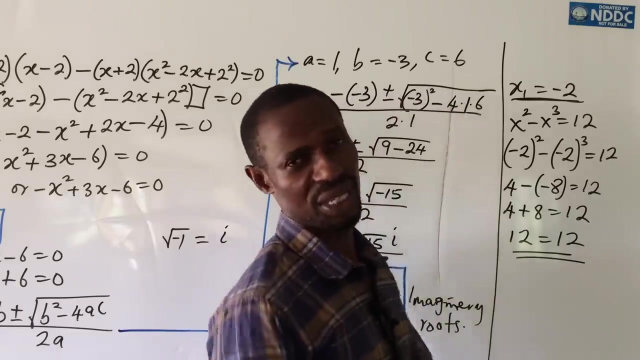 equal to 12. this will give us positive 4 minus. this will give us negative 8, the equal to 12.. here we're going to have here: 4 minus times minus will give us plus 8, equal to 12, and 4 plus 8 will give us 12 equal to 12.. as simple as a, b, c, okay. so this marked the end of 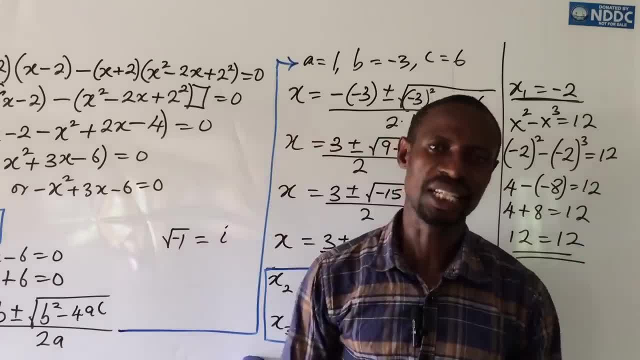 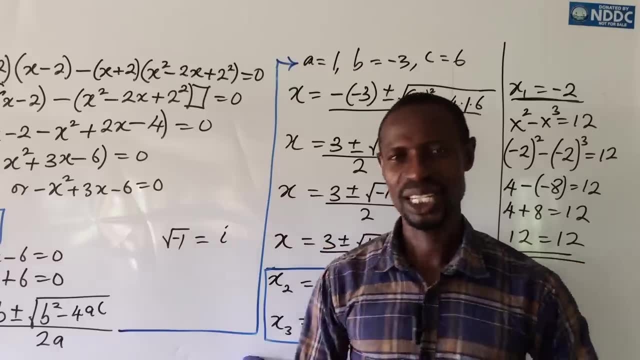 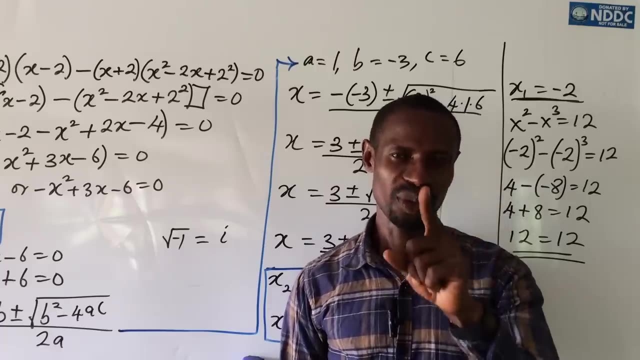 this only paid mathematical challenge or mathematical problem. i believe you enjoyed the solving. if you have learned something from this survey, drop a like and subscribe to my channel and i will see you in the next video. bye, bye. drop it in the comment section. do not forget to hit the like button and also do not forget to share. 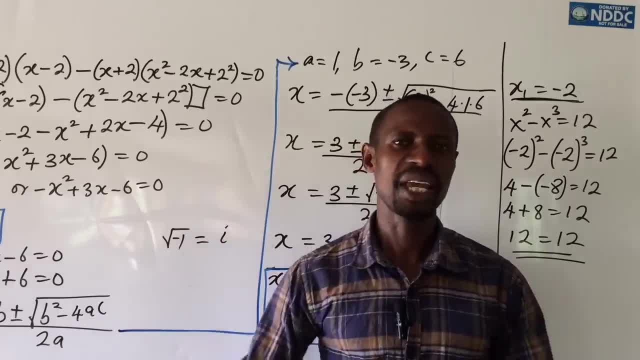 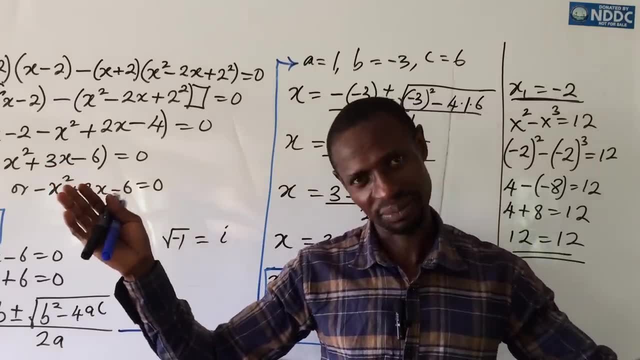 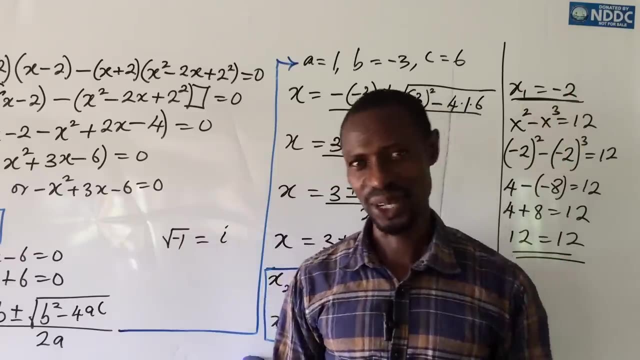 with family or friends. do not forget to also drop a comment. just leave a comment in the comment section below. okay, you can say thanks, jayce, for the work you're doing, or i love your ways of teaching, i love your method of explanation, or whoever be, i don't like the way you teach, i don't. 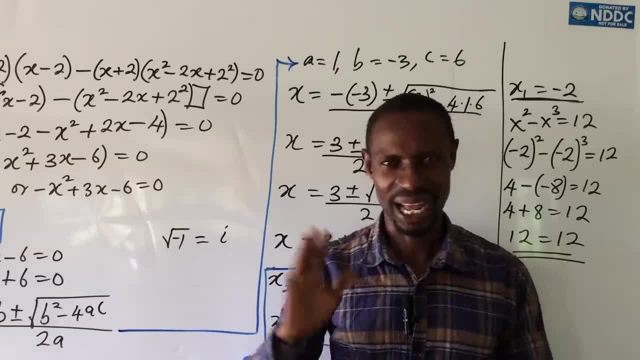 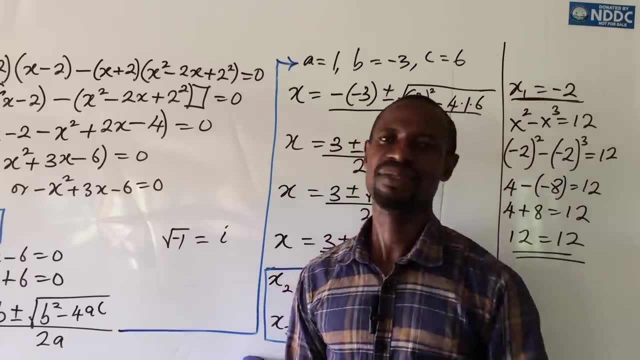 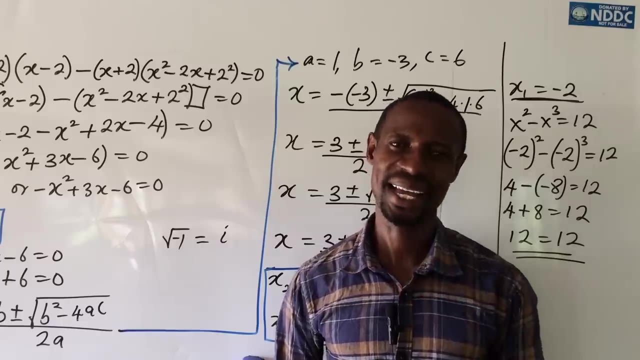 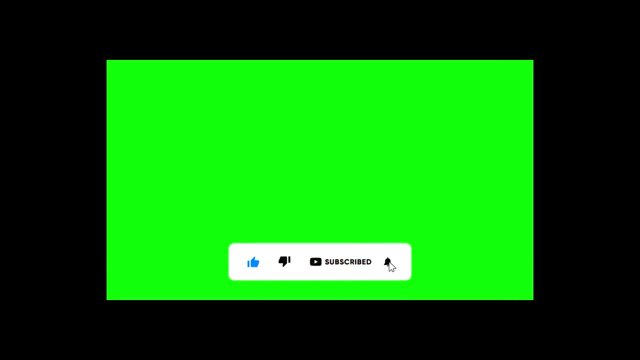 like the way you explain things. okay, drop it, okay, so that i can explain to you how to teach you know, make changes. all right, remember, this is all. i must tv and my name is jake's animal. i love you so much because you are always there, every one of us at all. i must tv. love you so much. bye for now.